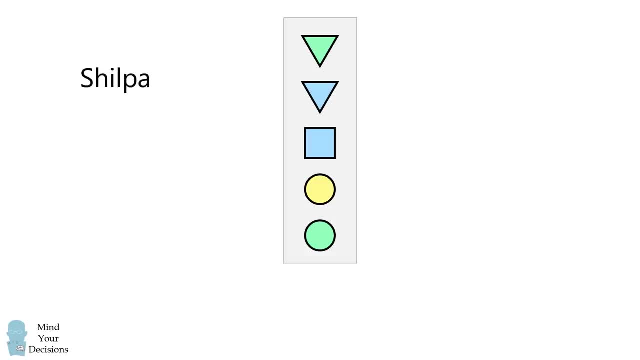 So how can we solve this problem? Shilpa was privately told the shape of the object. If she was told triangle, she would know it's either the green triangle or the blue triangle. If instead, she was told circle, then she would have known it was the yellow circle or the green circle. 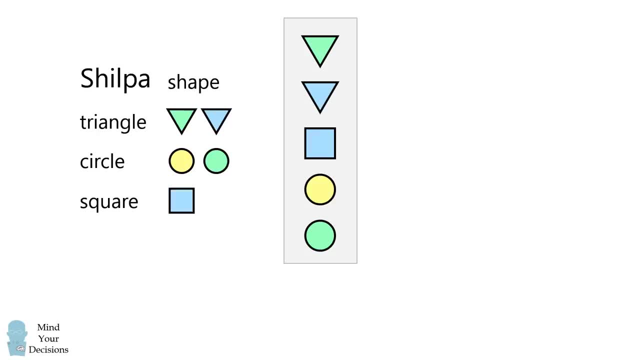 If she was told square, then she would have known it was the blue square. Similarly, Colin was privately told the color of the object. If he was told green, he would know it's either the green triangle or the green circle. If he was told blue, he would know it's either the blue square or the blue triangle. 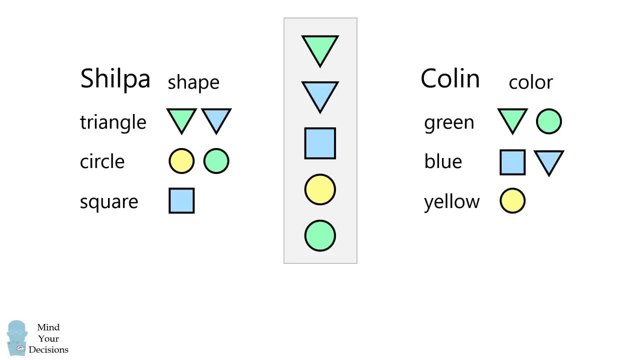 If he was told yellow, then he would have known it's either the green circle or the blue circle. If he was told yellow, then he would have known it's either the green circle or the blue circle. So let's analyze the first question. 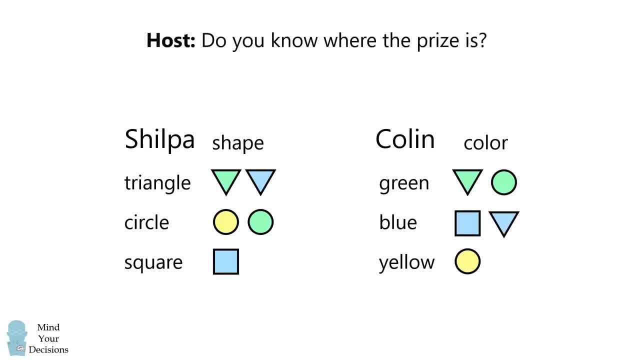 The host asked: do you know where the prize is? Both Shilpa and Colin are silent. So what does that mean for each person? Let's analyze Shilpa. If Shilpa had been told square she would have known. the prize is under the blue square. 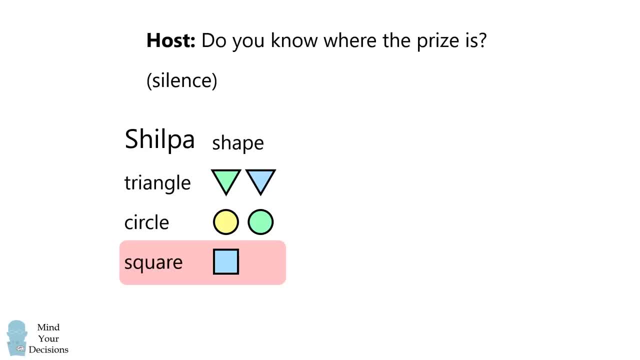 She didn't know this. she was silent, So we can eliminate that. Shilpa was initially told square. Now. similarly, if Colin had been told the color was yellow initially, then he would have known it's the yellow circle. But Colin was silent, so we can eliminate this. 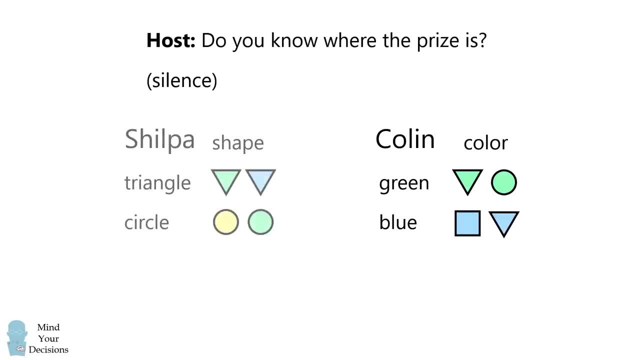 He was not told yellow initially. Now Shilpa has perfect logical reasoning. So she knows that since Colin was silent, Shilpa was silent. So she knows that since Colin was silent, Shilpa was silent. So she knows that since Colin was silent, Shilpa was silent. 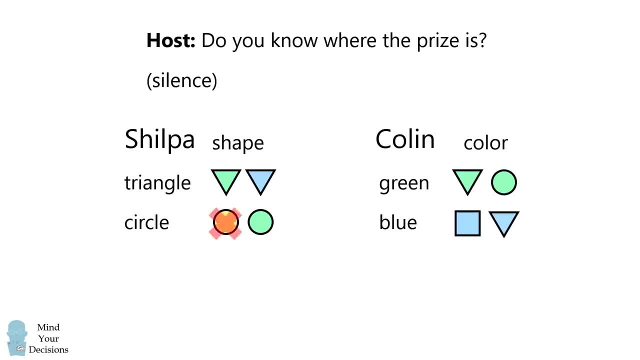 He was not told yellow initially, So Shilpa can eliminate the yellow circle as one of her options. Similarly, Colin knows that Shilpa was not told square initially, So he can then eliminate the blue square from his options. So now we go to the second stage of reasoning. 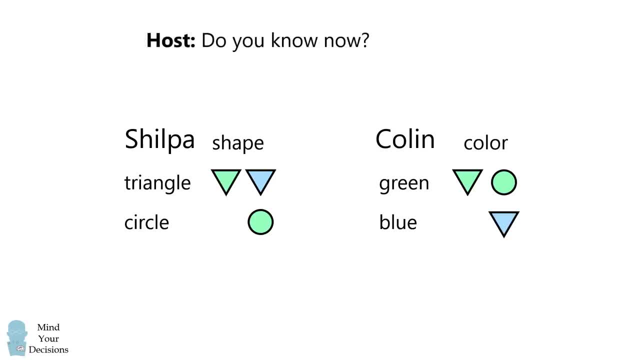 Now the host asked: do you know? now, Once again, they are both silent. Once again, they are both silent. So we can repeat this type of logical reasoning At this stage. if Shilpa had been told circle initially, the only option would be the green circle. 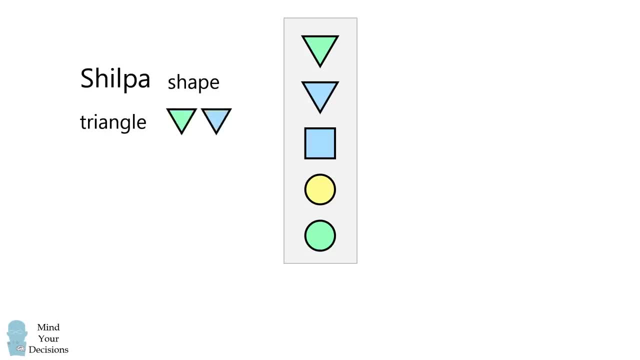 If she was told triangle, she would know it's either the green triangle or the blue triangle. If instead she was told circle, then she would have known it was the yellow circle or the green circle. If she was told square, then she would have known it was the blue square. 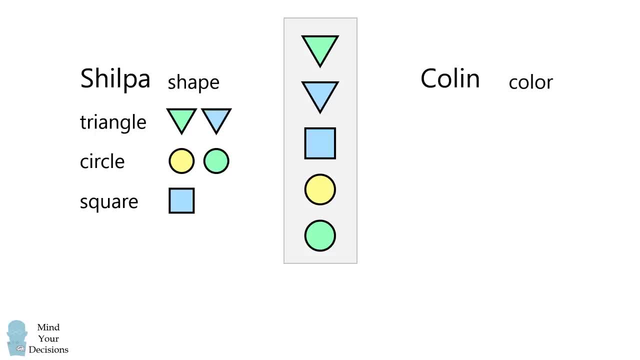 Similarly, Colin was privately told the color of the object. If he was told green, he would know it's either the green triangle or the green circle. If he was told blue, he would know it's either the blue square or the blue triangle. 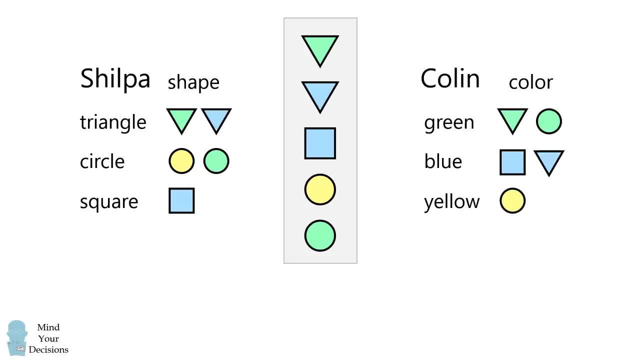 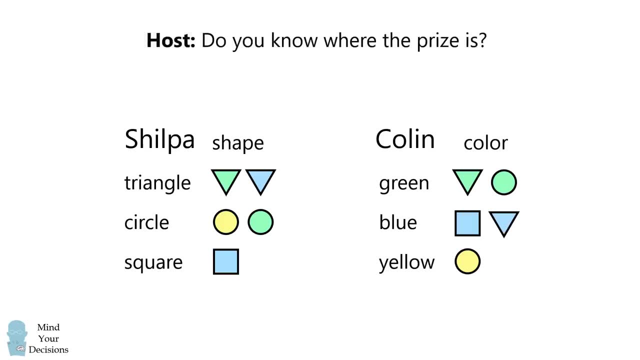 If he was told yellow then he would have known it was the yellow circle. So let's analyze the first question The host asked: do you know where the prize is? Both Shilpa and Colin are silent, So what does that mean for each person? 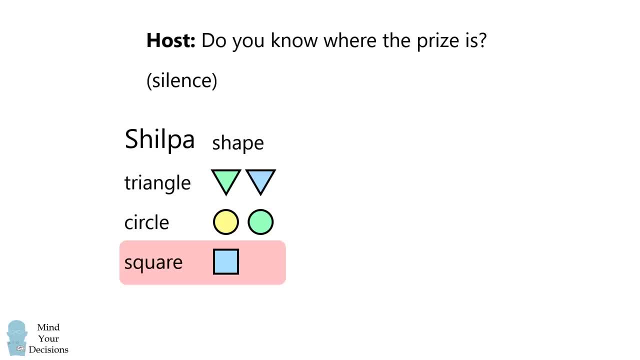 Let's analyze Shilpa. If Shilpa had been told square she would have known the prize is under the blue square. She didn't know where the prize is under the blue square. If Shilpa didn't know this, she was silent. 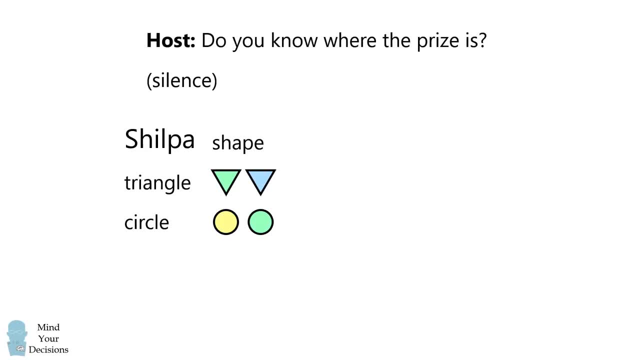 So we can eliminate that. Shilpa was initially told square. Now. similarly, if Colin had been told the color was yellow initially, then he would have known it's the yellow circle, But Colin was silent, so we can eliminate this. He was not told yellow initially. 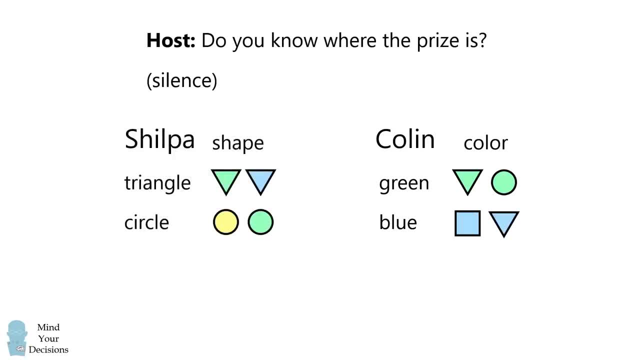 Now Shilpa has perfect logical reasoning. So she knows that since Colin was silent, he was not told yellow initially. So Shilpa can eliminate the yellow circle as one of her options. Similarly, Colin knows that Shilpa was not told square initially. 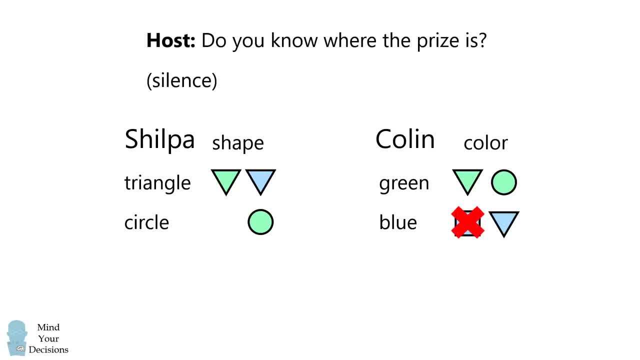 so he can then eliminate the blue square from his options. So now we go to the second stage of reasoning. Now the host asked: do you know? now, Once again, they are both silent, So we can repeat this type of logical reasoning. 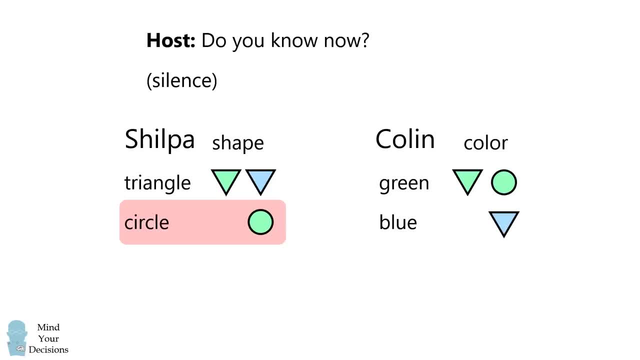 At this stage. if Shilpa had been told circle initially, the only option would be the green circle. By this stage she would have known where the prize was. She was again silent, So this is not what she was told initially.